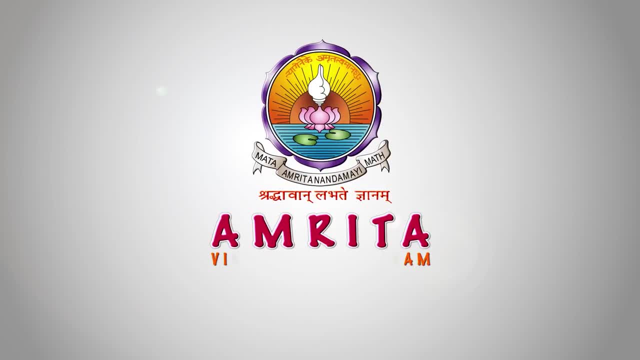 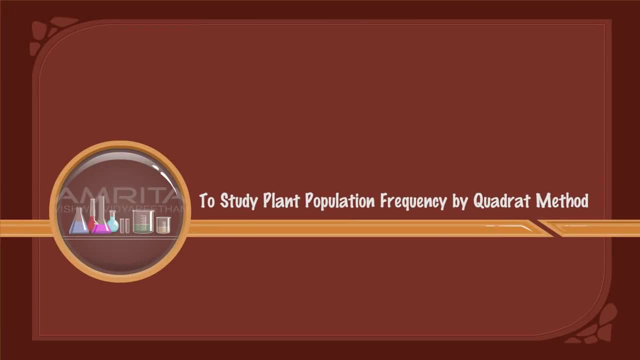 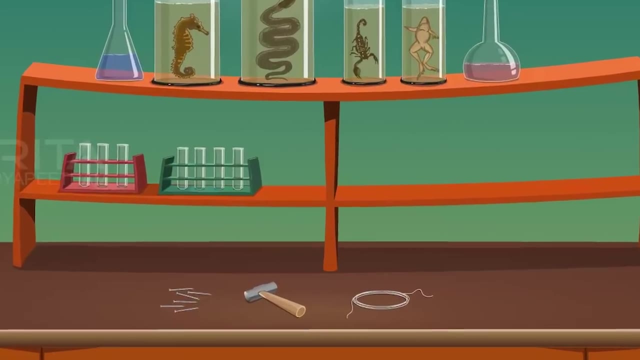 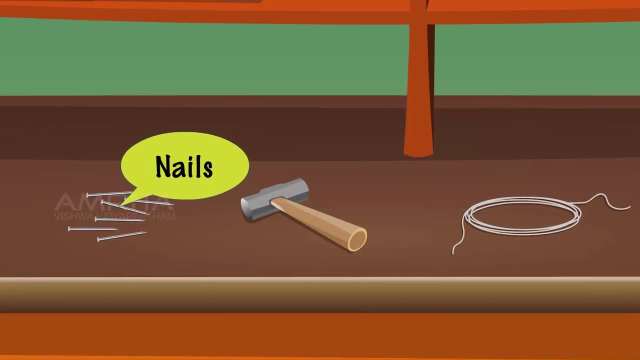 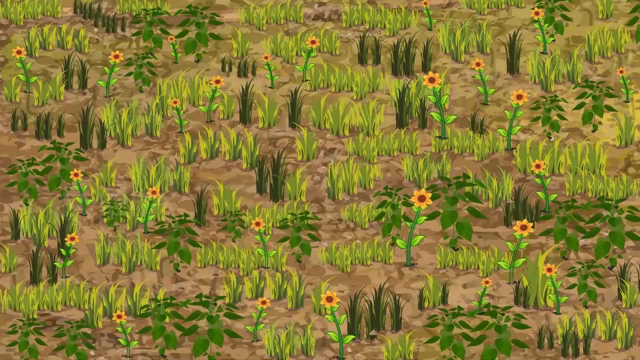 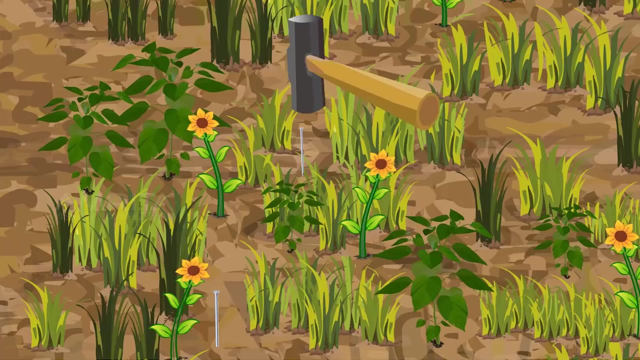 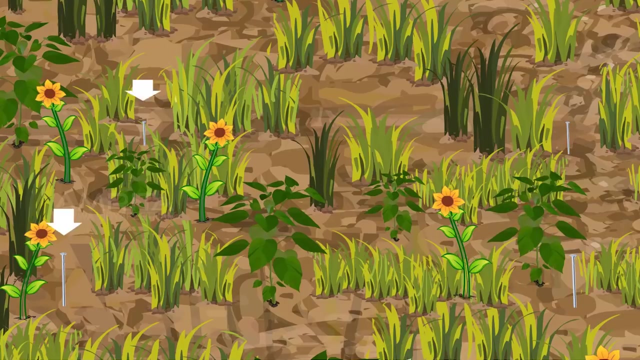 To study Plant Population Frequency by Quartret Method. Materials required: Nails, A hammer and a thread. Procedure In the selected site of study: hammer the nails firmly in the soil without damaging the vegetation. Fix four nails to make a square. Tie each end of the nails using a thread to make a quadrant. 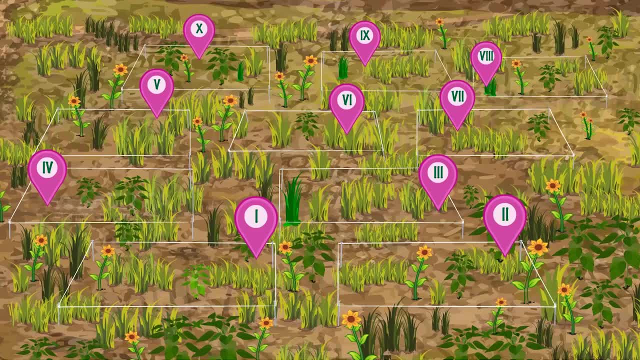 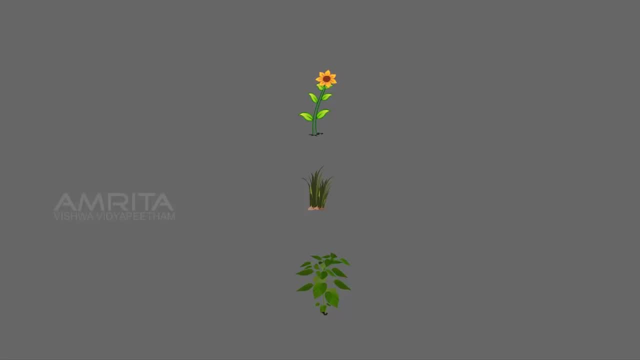 Similarly, make nine more quadrants randomly in the site of study. Select the plant species for study of the Population Frequency. Observe the presence of species at the site портив. Did you know that there are nine types of plants in a snaps? 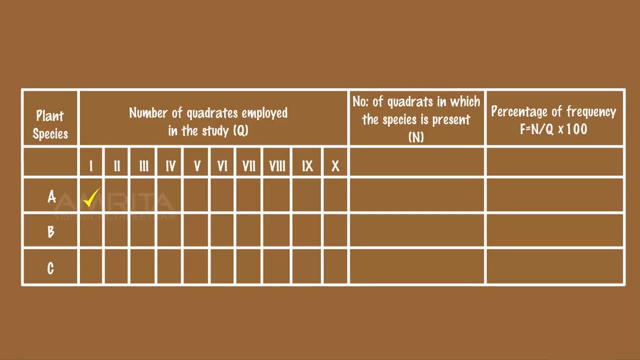 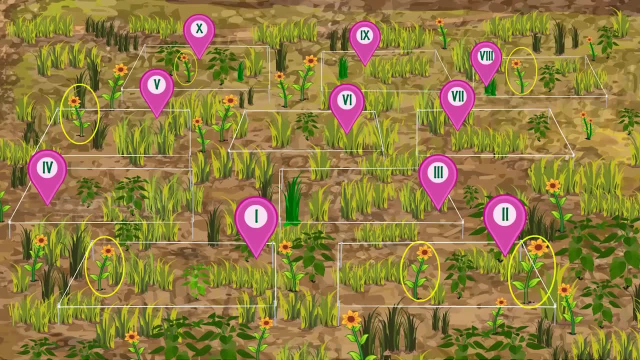 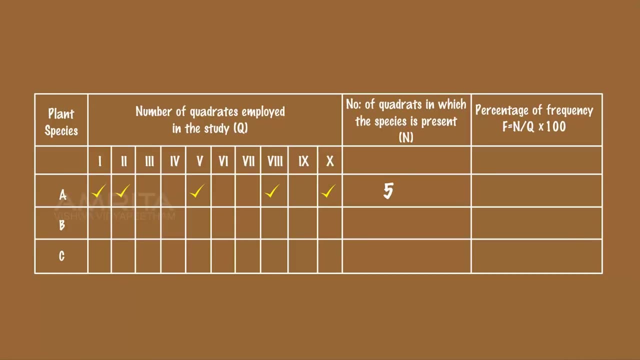 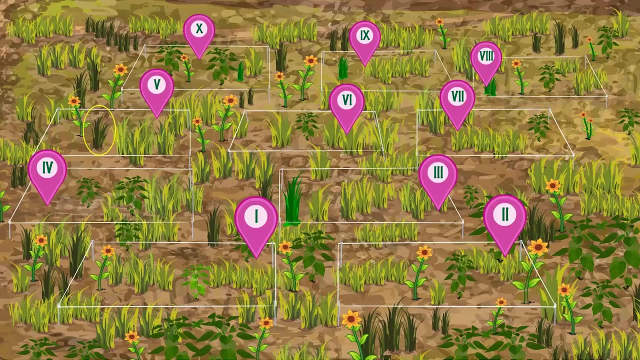 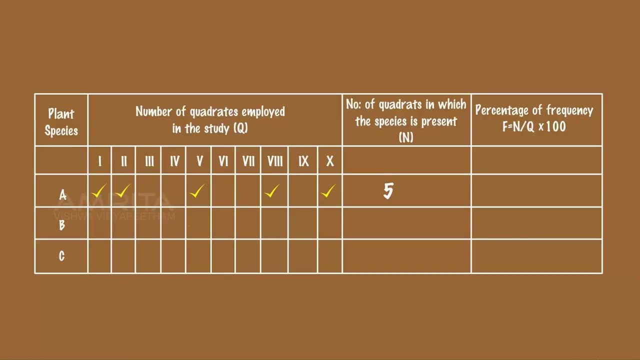 Species A in the first quadrant and mark it in the table. Similarly, check for the presence of Species A in the quadrants respectively and record the data in the table. Observe the presence of Species B in all quadrants and mark it in the table. 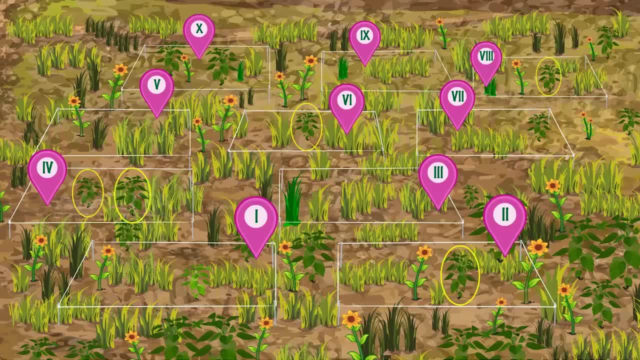 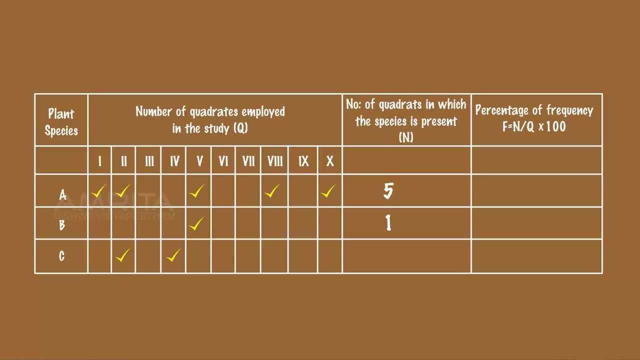 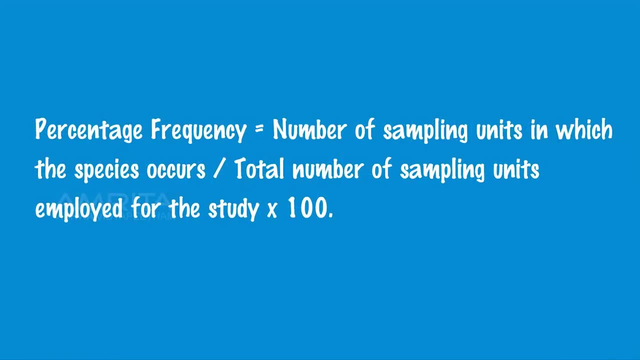 Repeat the same procedure for Species C and record the data in the table. We can calculate the frequency of the plant population by this equation. Percentage frequency is equal to number of sampling units in which the species occurs, divided by total number of sampling units employed for the study into hundred. 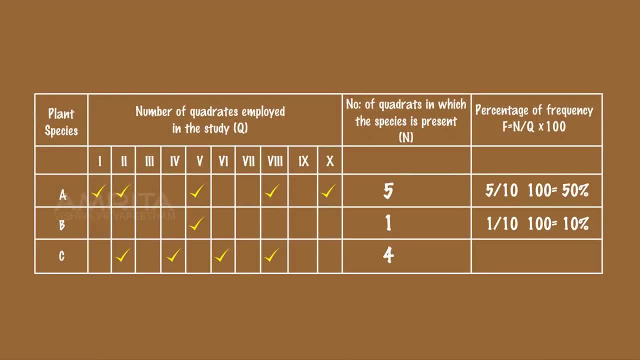 Frequency value indicates the number of times a plant species is present in the sampling unit present within a given number of sample quadrants.